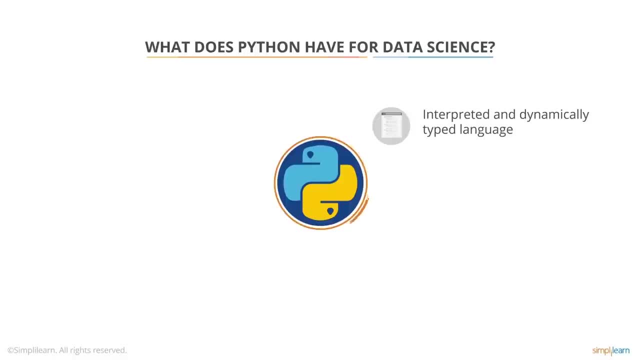 Python is an interpreted, dynamically typed language with a precise and efficient syntax, and is renowned for its ease of use to analyze, visualize and present data. Python has an extensive library with built-in modules providing easy access to system functionalities, which not only improves accessibility but also provides standardized 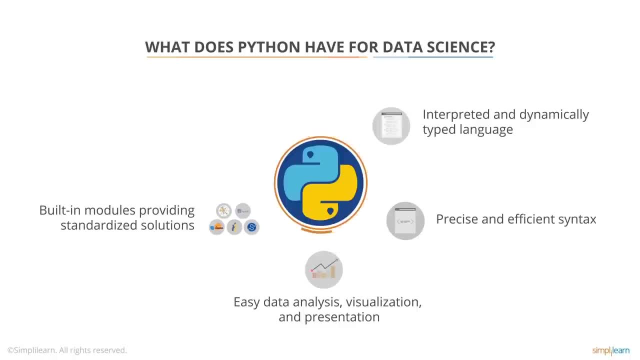 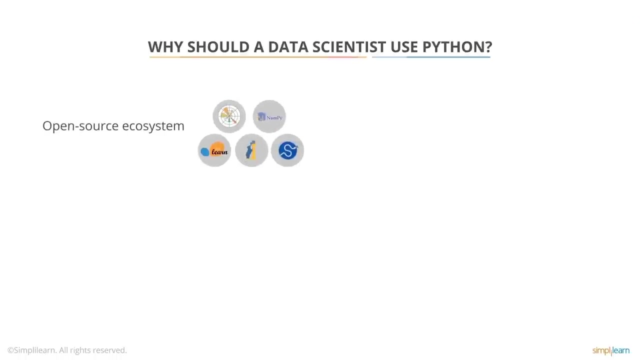 solutions for everyday programming challenges. By taking away platform-specific requirements and replacing them with platform-neutral APIs, modules in Python libraries encourage users to make programs portable. Why should a data scientist use Python? Apart from being an open-source ecosystem, Python and most of its incredible libraries are platform-independent, so you can run this. 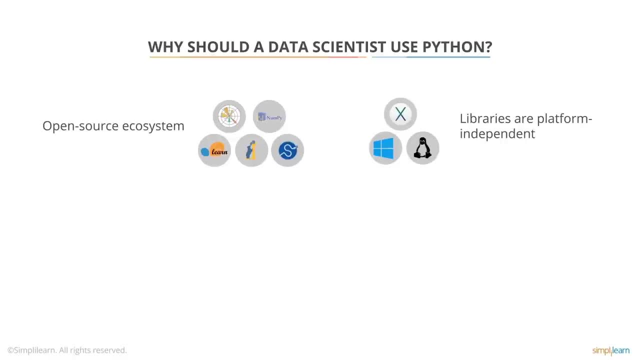 notebook on Windows, Linux or OS X without a change. Python is part of the winning formula for productivity, software quality and maintainability at many companies and institutions around the world. Python is one of the leading technologies used widely in academic circles and industries. 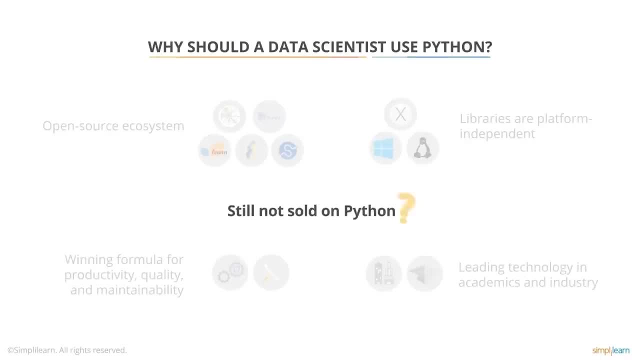 because of its flat learning curve, Still not sold. Want to learn more about Python? Then here's some proof. Case study: Forestwatchcom, a weather report accuracy rating service, is a 100% Python solution, using it in all its components- the front-end, back-end, as well as the performance-critical. 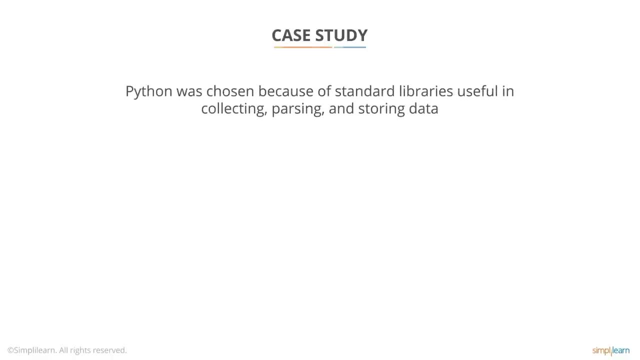 portions. Python was chosen to develop this solution as it comes with many standard libraries useful in collecting, parsing and storing data from the web. Python is impressive as an object-oriented, rapid-application development language. One of Python's key strengths lies in its ability to produce results quickly without 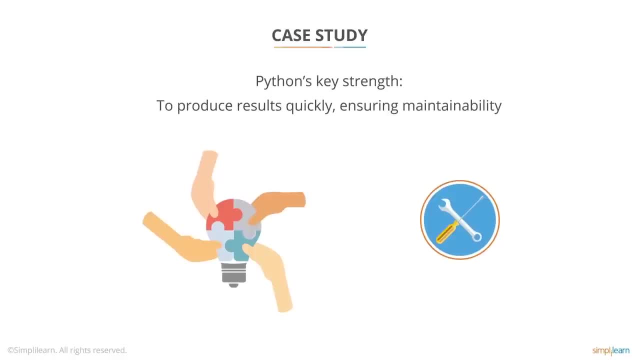 sacrificing maintainability of the resulting code Because of the clean design of the language. refactoring the Python code was also much easier than in other languages. Moving code around simply requires less effort. Forecastwatchcom was made possible because of Pythoncom. For more information, visit wwwforecastwatchcom. 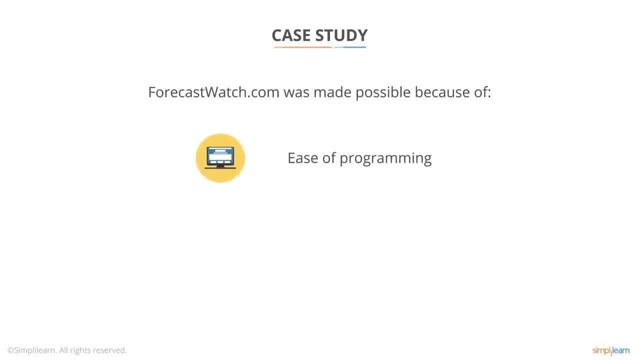 For more information, visit wwwforecastwatchcom. Question: Are there any other tools you'd like to see in the next three years That this new video will give you a better explanation of Python? Answer: According to a survey by the Association for Computing Machinery, ACM, posted on javaworldcom, Python has surpassed Java as the top language used to introduce US students to programming and computer science. 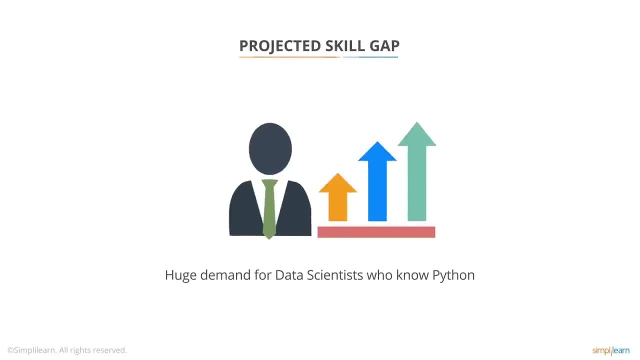 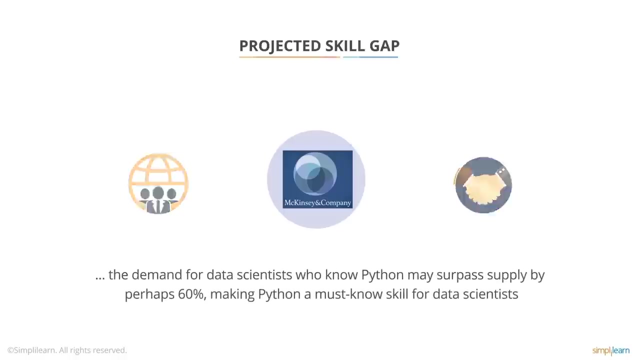 Projected skill gap. There is also going to be a huge demand for data scientists who know Python. McKinsey & Company, a trusted advisor and counselor for many of the world's most influential businesses and institutions, projects that by 2018, the demand for data scientists who know Python may surpass supply by perhaps 60%. 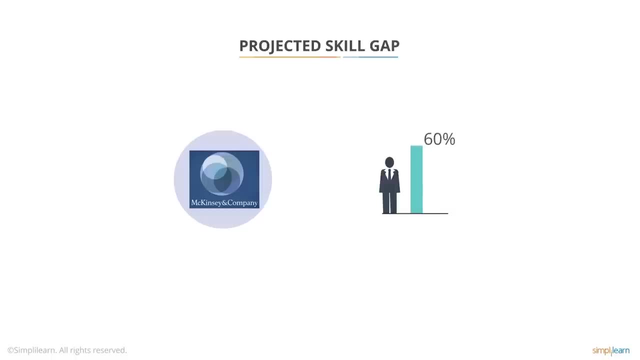 making Python a must-know skill for data scientists. Forbescom mentions that the demand for Python programmers in big data-related positions increased by 96.9% and that the demand for Python programmers in big data-related positions increased by 96.9% in 12 months. 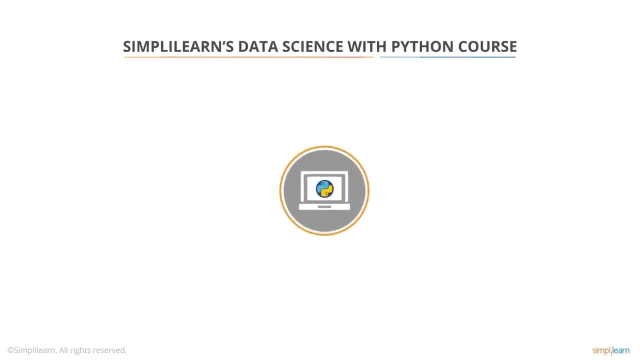 Simply Learn's Data Science with Python Training is designed to ensure that you are ready for any assignment in data analytics And you know what You will also get to work on real-life industry projects spanning over three months to get that vital hands-on experience you're looking for. 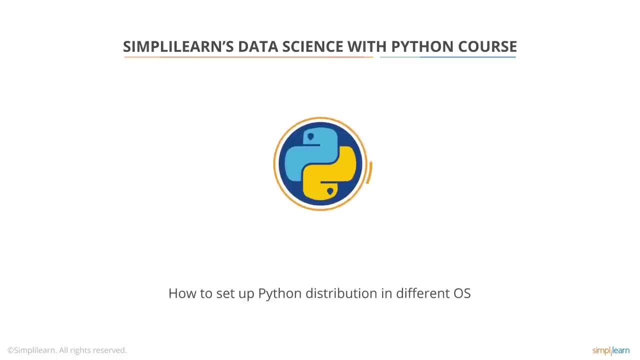 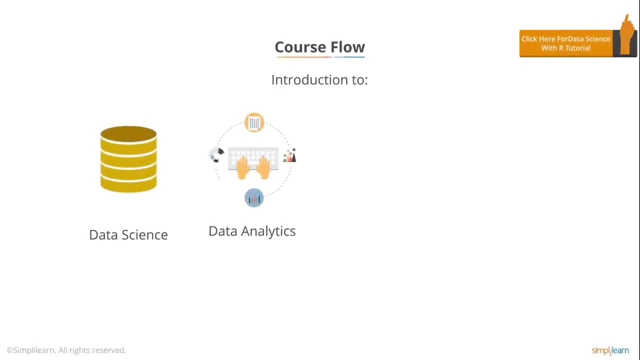 Apart from this, you will also learn how to set up a Python distribution in different operating systems, master all the Python functions and acquire an in-depth understanding of machine learning techniques and natural language processing with Python. The course flows as follows: You start with an introduction to data science and data analytics. 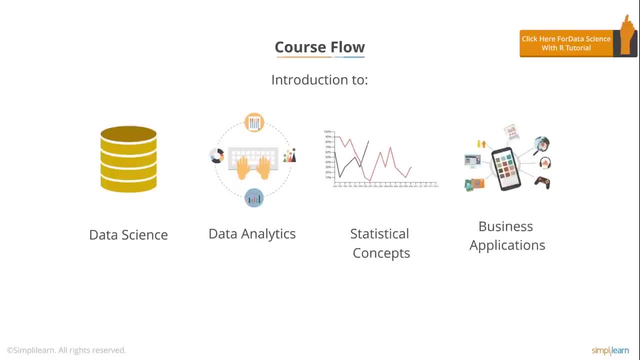 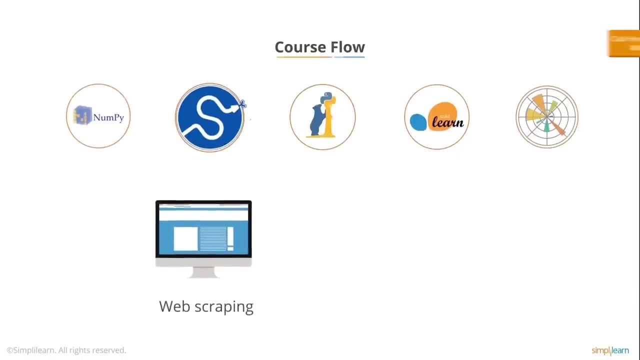 and statistical concepts and business applications. Continue on to Python environment setup, then the Python libraries NumPy, SciPy, Pandas and Matplotlib. You will also learn about web scraping and Python integration with Hadoop Once you've gone through all the lessons.